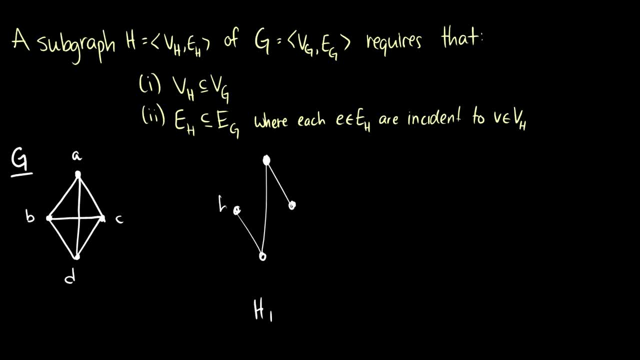 H is a subgraph of G, So H1 is a subgraph of G, because we've kept all the vertices but we're just missing a few edges. So it's edge set BDDAAC. So H1 is in the edge set of G and the vertex set ABCD is in the vertex set of G. So what's another? 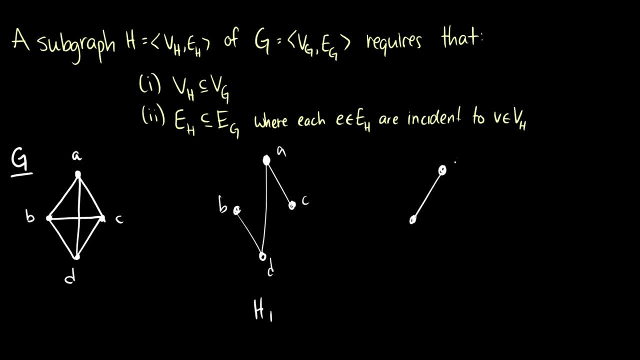 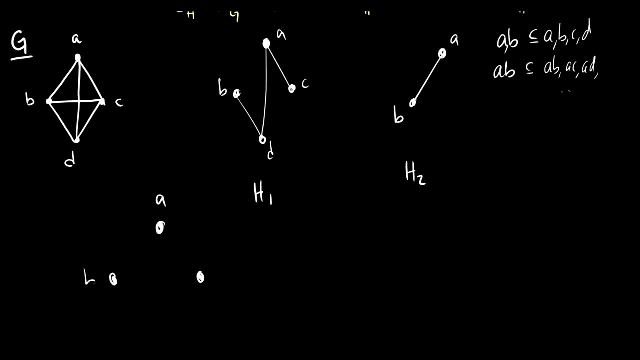 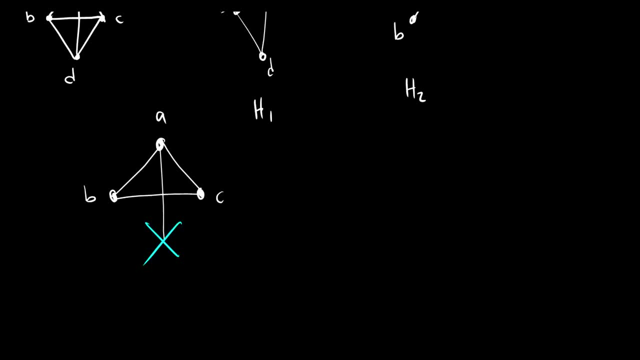 This is why the edges must be incident to the vertex set, because we need a D there, In fact. another thing that's not a subset is if I said, okay, so there's ABC, but then we have this extra vertex- we'll put it here- called E. that is not a subset, because E in R, we'll call this. 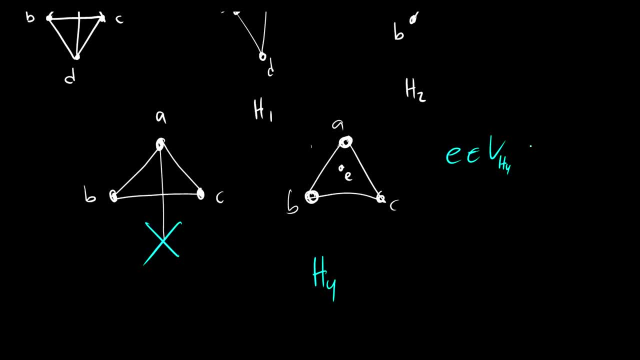 H4.. E in V of H4 is so this vertex E is in H4, but E is not in our regular graph G, which we should say VG. So clearly not a subgraph, because we added a vertex. A spanning subgraph are all the subgraphs where the vertex set is the same. So if we're 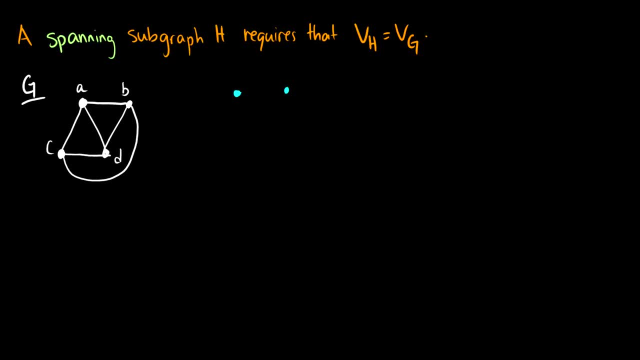 For instance, if we want a spanning subgraph of G, that means that we have to keep A, B, C and D. Then we can do whatever we want with the edges. For instance, this graph here, H1, this is a spanning subgraph of G because we have all the vertices. We don't need to keep the edges. So that is a spanning subgraph of G. What is another spanning subgraph of G? 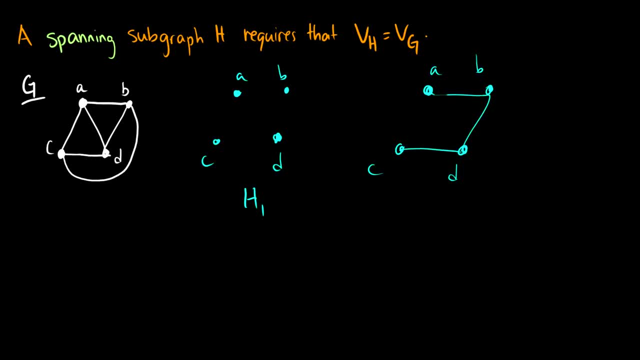 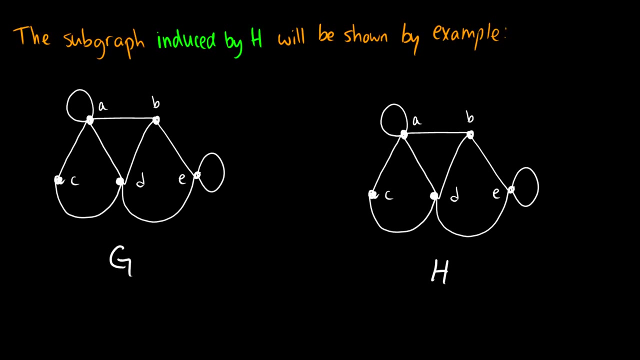 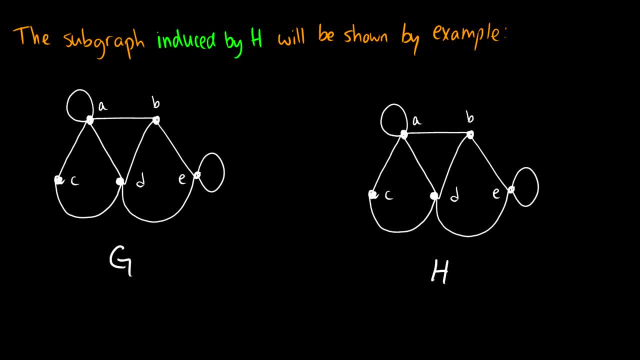 an example of this. So here's what we do: When we induce a graph, we remove an edge. So, for instance, let's remove the edge C. And when we remove an edge, we just remove only the edges. Crazy, We only remove the edges that were incident to that vertex. So because we removed C, we only removed CD and CD. 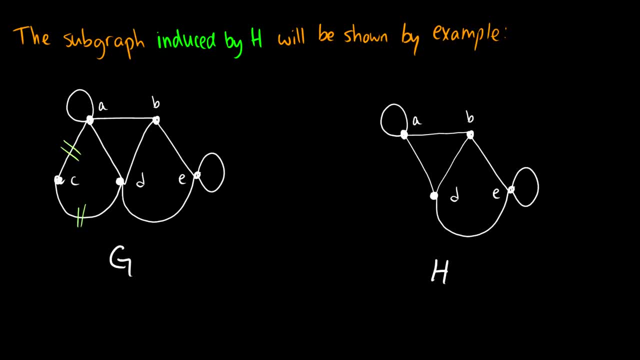 You cannot remove any other edge. When we induce a graph, we remove only the edges incident to the vertex we removed. So, for instance, if we remove E here- let's say we take E- well then we have to remove this edge, we have to remove the edge from E to B and we have to remove the edge from E to D. So we have to take all of these out. So H, B, C and D. 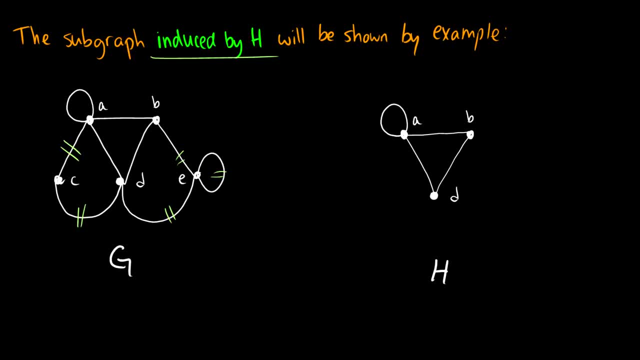 is an induced subgraph of G. So how can we write this in notation? Well, we'll get to that, But here's a question: How many spanning subgraphs are also induced? So what does that mean? How many subgraphs of G- where all the vertices are kept- are also induced? Well, here's an answer. 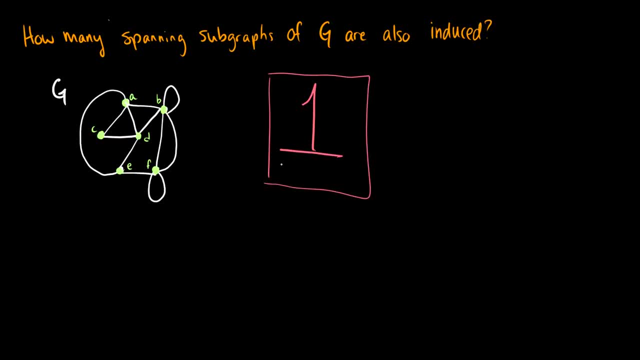 One For every graph. there is exactly one subgraph. that is spanning and induced. Why? Because spanning says all vertices. Induced says remove vertex Adjacent edges. Well, incident edges, That would be the correct term Incident edges. So the one case where spanning is induced is when the induced says remove nothing. 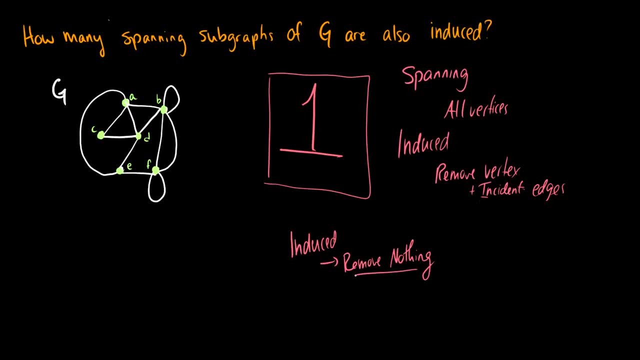 And that is the only scenario where the spanning subgraph is the induced subgraph. So that's a fun little question And I put this right here just as an example. So the spanning subgraph G: well, if we remove an edge- let's say hypothetically we removed AE- it is no longer induced because we removed an edge without removing its vertex. 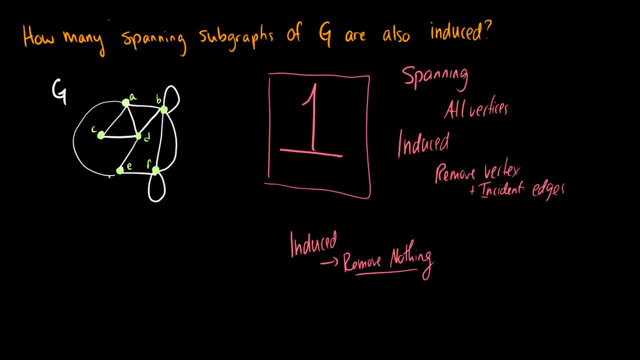 So in an induced subgraph you cannot just remove an edge without removing its vertex. You can only remove edges if it is touching a vertex you removed. So the graph is just a nice visual example for you to figure things out on your own. if you read a slide and like, hey, I'm going to figure that out first, 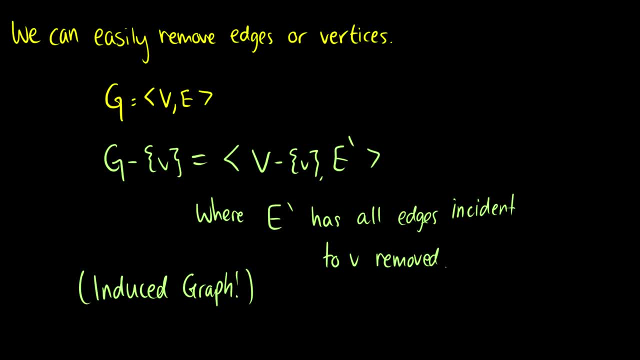 So maybe I tricked you. It's only one. So how do we write this? Well, if we have a graph, G is equal to VE. we just write G minus the set containing whatever vertex, And this is just equal to the graph V minus that vertex, with a new edge set: E, prime. 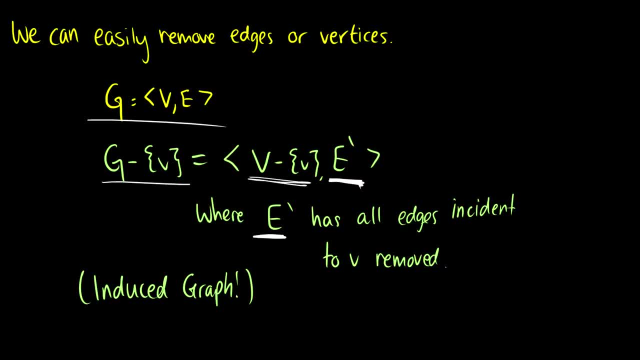 And this E prime has all the edges incident to V removed. So, for instance, if we have, say, a graph here and this right here is our V, we have an edge. We'll call this E1, E2.. So V, we'll call this AB. 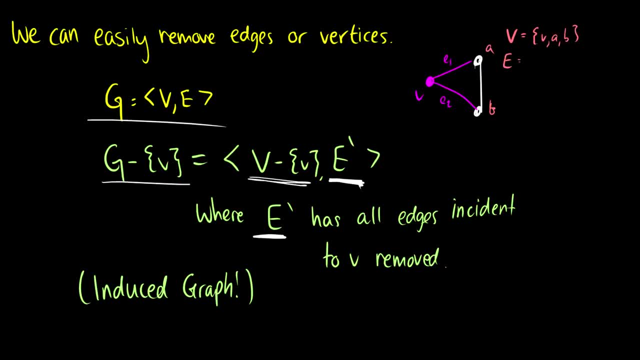 V has the edges V, A and B, And E has the edges E1,, E2, and we'll call this E3.. Then V minus V or V minus little v is just going to be the vertex set AB. 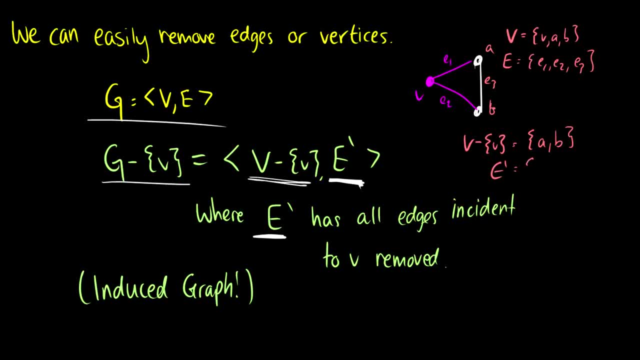 So we subtracted V from it And then this E prime here is just going to be E And this is just going to be E3, because E1 was touching V and E2 was touching V. So we remove those and we just get left with A touches B through E3. 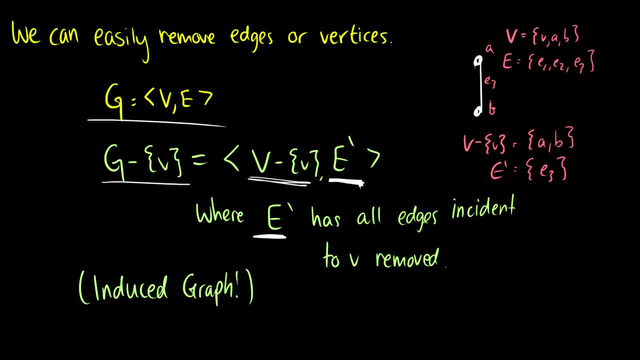 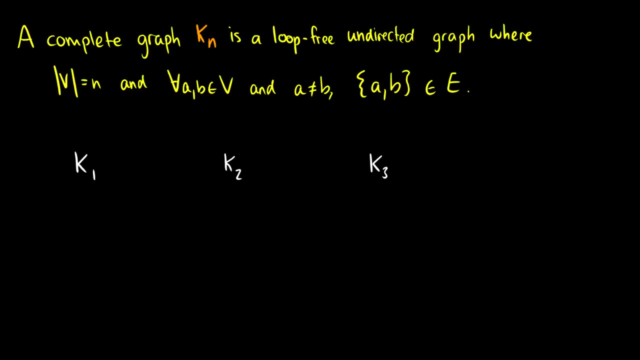 So that is how we write graphs: that we induce by removing specific edges. So this is an induced graph. Okay, what is a complete graph? A complete graph which we'll always say k little n is a loop-free, undirected graph. 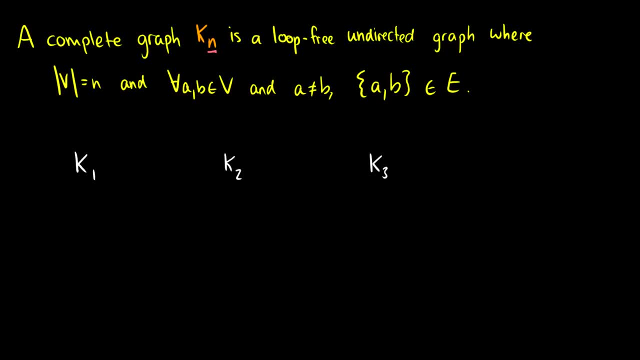 where the amount of vertices is denoted by this number, n, And for all vertices that are not equal to each other, there is an edge between them. So for all AB and V and A is not equal to B, the set AB is in edges. 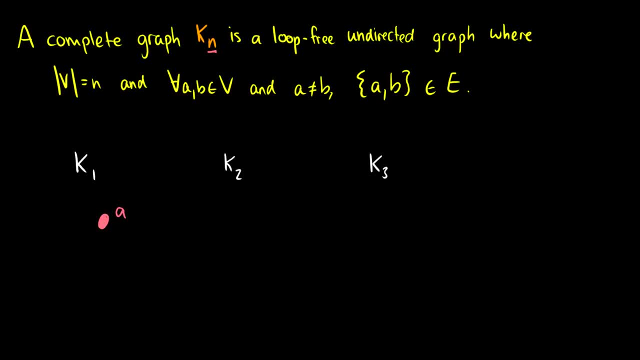 So, for instance, K1, we have this vertex A And there is an edge between all vertices. Okay, K2, we have two vertices here And we need to connect them to each other, So that is K2.. In K3, we have three vertices. 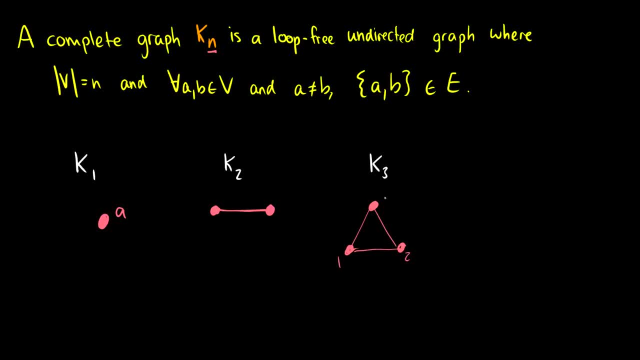 And they all have to be connected to each other. So if we have 1,, 2, and 3,, 1 has to be connected to 2, and 1 has to be directly connected to 3.. Same with 3 with 1 and 3 with 2.. 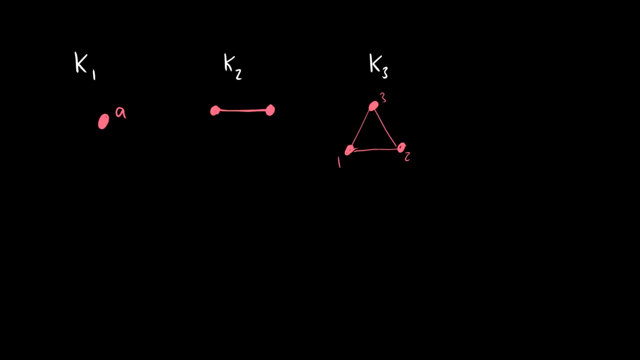 And 2,, 1,, 2, 3.. Let's take a look at K4.. K4.. Okay, we got four vertices here, So this top left one has to be connected to bottom left, bottom right, top right. 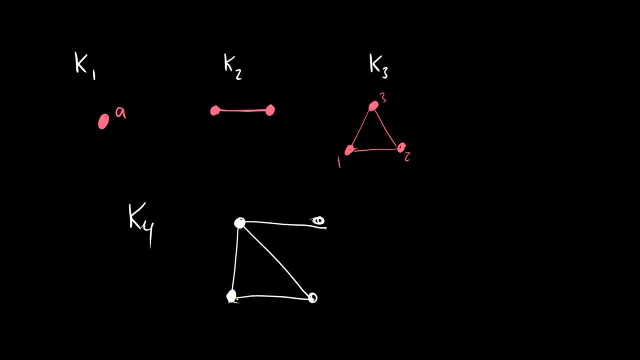 Bottom left has to be connected directly to all other vertices. So we can do this here And let's loop this around. We could cross it if we want, so let's just cross it for now. And this bottom right vertex has to be connected to all others. 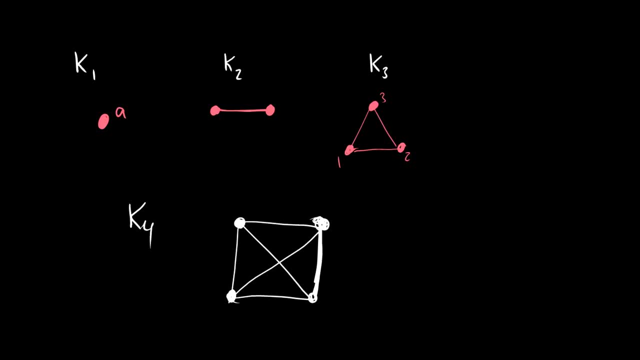 So we'll just draw that one. So that is the complete graph K4.. The reason I drew it so that way this middle was looped around is because I like it to be planar. But we'll discuss planarity a little bit later. 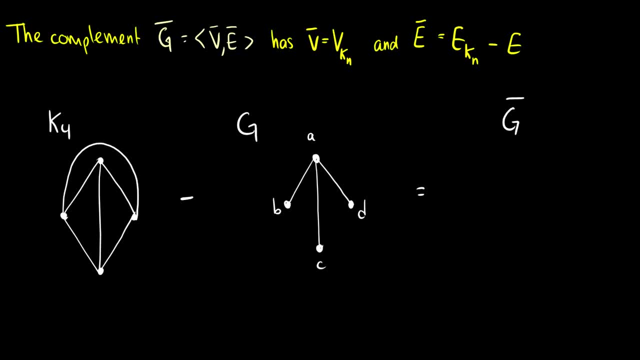 So that's a complete graph. A complement is essentially the same vertex. So if we have the complement which we'll call V bar, E bar or G bar, it means that the vertex set is essentially the vertex set of the complete graph. 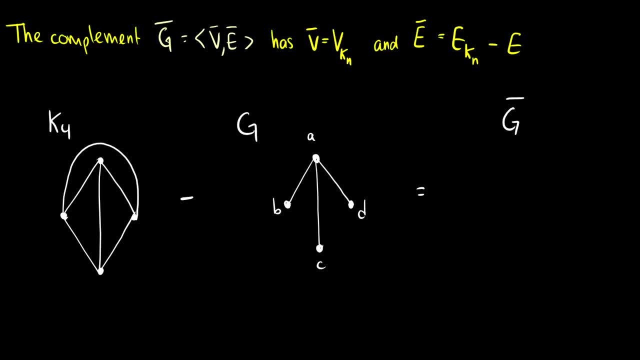 And the edge set is going to be all the edges in the complete graph minus the edges in the original graph G. So, for instance, here's K4.. It's the graph we just did. on the other page It's just shaped as a diamond. 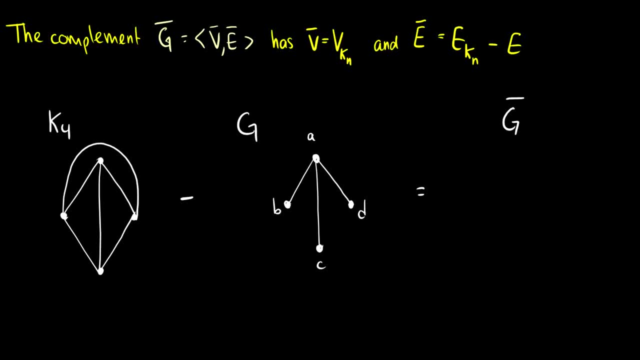 So each vertex is connected to all other vertices. So each vertex is connected to all other vertices. And here's our graph G. So we should probably label these A, B, D and C. So in G bar we keep the same vertices. 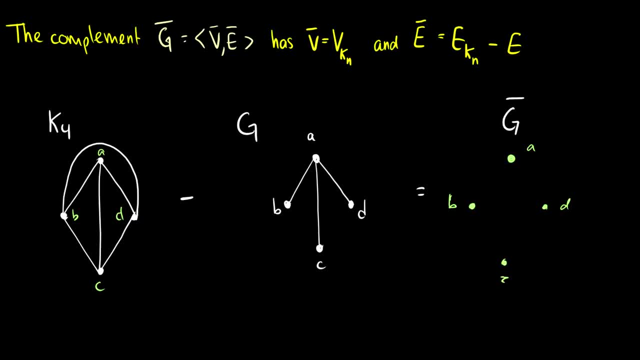 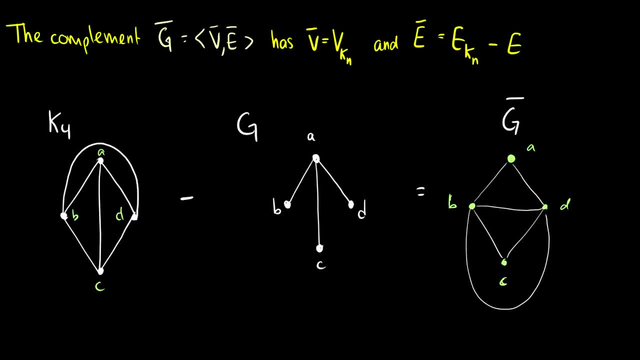 And then we'll loop this around here, But we subtract all of the edges in G, So we remove the edge between A and B. We remove the edge between. Sorry, This graph was wrong. It should have looked like this: Okay. 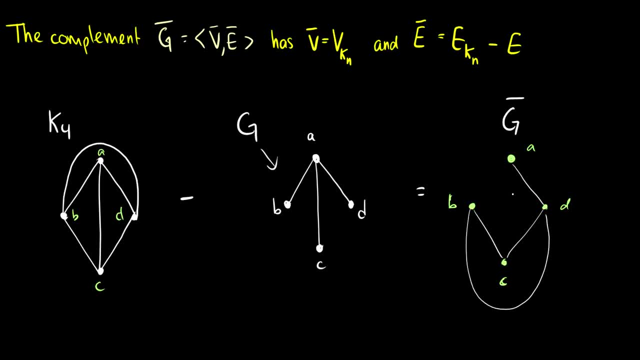 So we remove the edge between A and B, We remove the edge between A and C And we remove the edge between A and D. So now is the complementary graph of G, Basically all the edges it didn't have, that it could possibly. 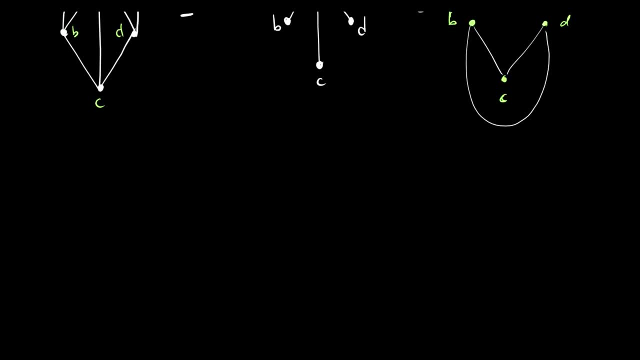 have it now has. So here's a question. Suppose our graph. let's be a little bit more formal about this. I do remember this question from a textbook. So we have the graph: G is equal to VE and we have V. the number of edges in V is equal to little v and the number of edges in E is equal to little. 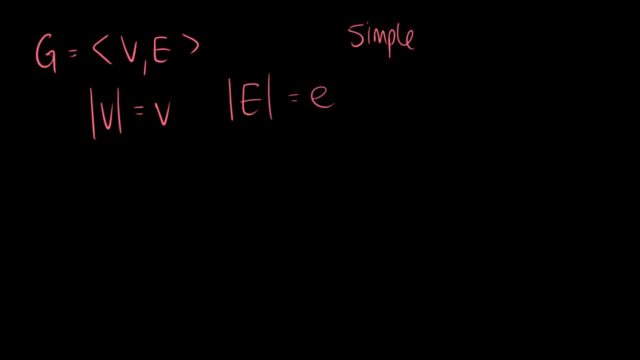 e. Of course this is going to be simple. So here's the question: What is the number of edges in E bar? Okay, well, we have. G is equal to V bar, E bar. Well, really, we know that V bar. 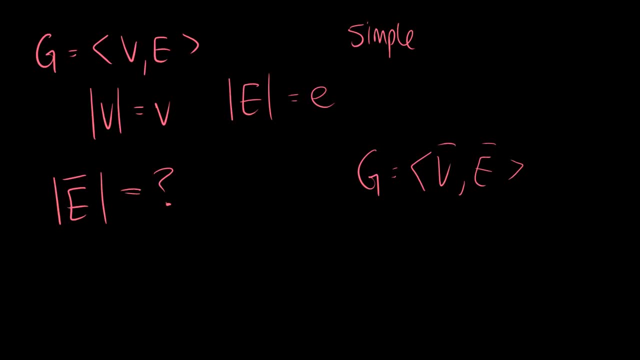 is the number of edges in E bar, and we know that V bar is. the number of edges in E bar is the same thing as V, because it has to have all the vertices. still, The complement really just switches the edges from off to on and on to off. So here's the thing: How many edges? 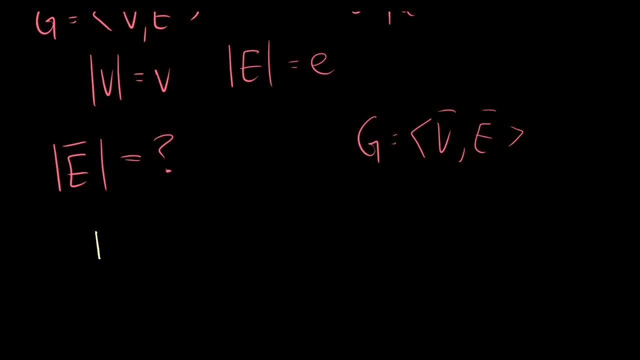 are there total. So we went over this in the last video: The total possible edges in KN. so that's going to be V choose 2.. So you take all the different vertices and you say, okay, for each two I choose, I want to put an edge between them, And then we're going to subtract. 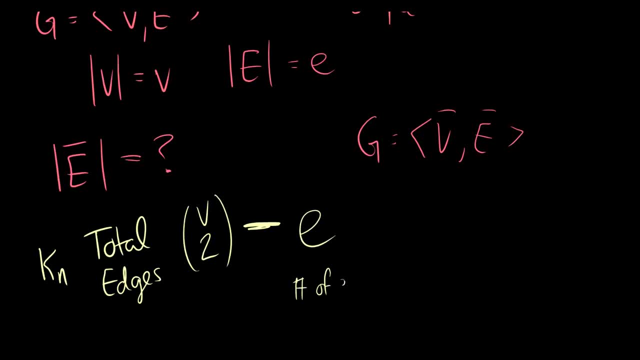 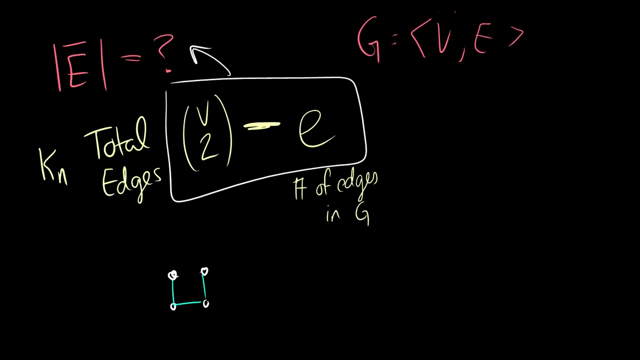 the number of edges in G. So this is number of edges in G, So this is how many edges there are in the complement of G. So, for instance, let's take a look at this one. So we have three edges here. So probably just draw it. 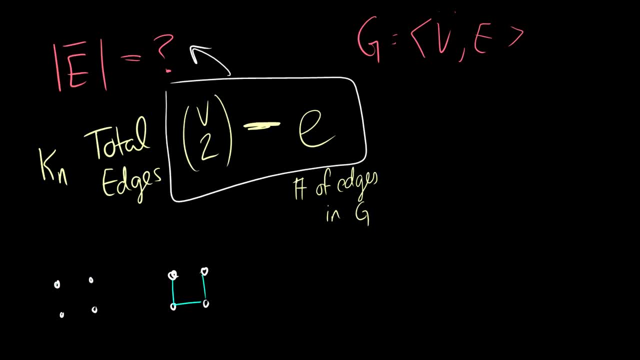 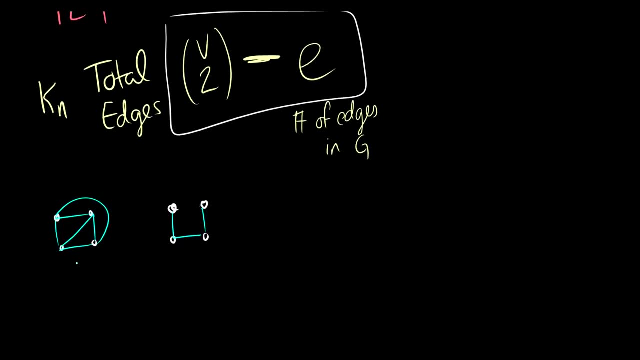 out K4.. So we'll do K4 like this: 1,2,3.. 4,5.. 6.. So K4 has six edges. So for choose to, because we have four vertices and we choose to, which is just four times three over two, which is six. 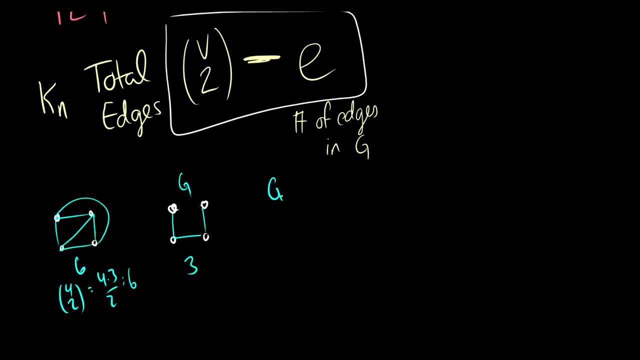 Here is our G. So we see three edges here. So this means that G complement should have 6.. 6 minus 3 equals 3 edges. so that means it should have this one, it should have this one and it should have this one, which is right. So by example, we've shown that, yes, this works. 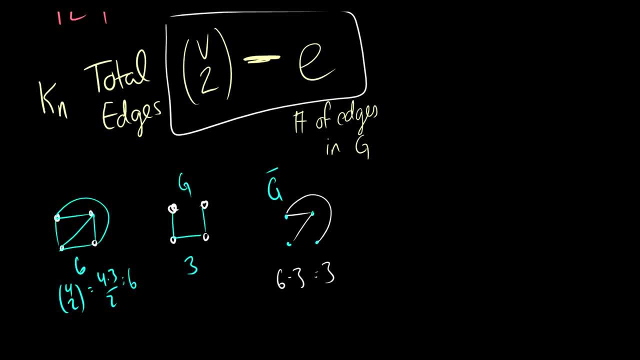 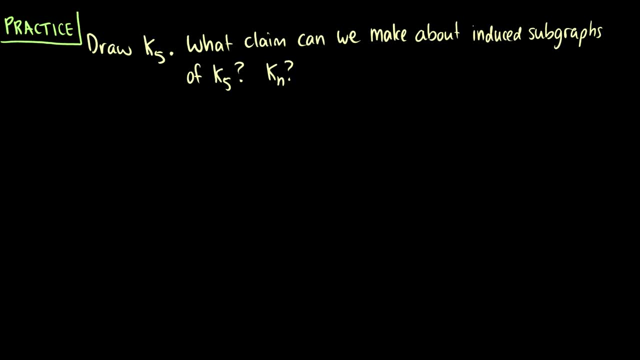 and, of course, you can always verify your conjectures with examples. That's a great thing to do. So that is complements, and let's do some practice. I want you to draw k5, so take a piece of paper, do it in your head, draw k5. Okay, what does k5 look like? 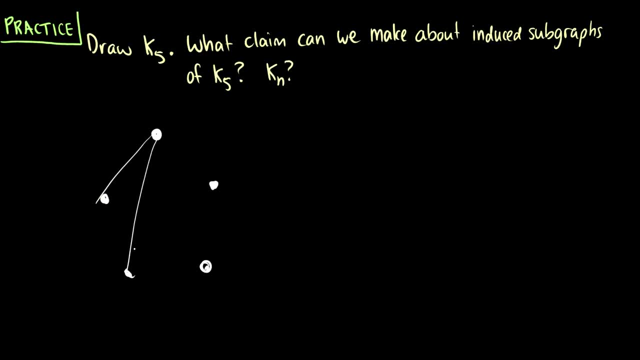 Well, we have five vertices and each one has to be connected to all the others. I'm going to do it in light green. Okay, so that goes to four edges, this one goes to four edges, this one goes to four edges and that one goes to four vertices. When saying edges, I meant to say vertices. 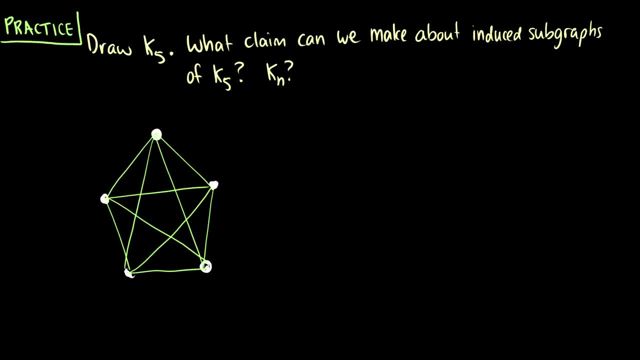 Okay, so each vertex goes to four other vertices. Got a nice beautiful star pattern here. So what happens when we try to make an induced subgraph? Remember what an induced subgraph is. An induced subgraph is: when we take one edge, we delete it. 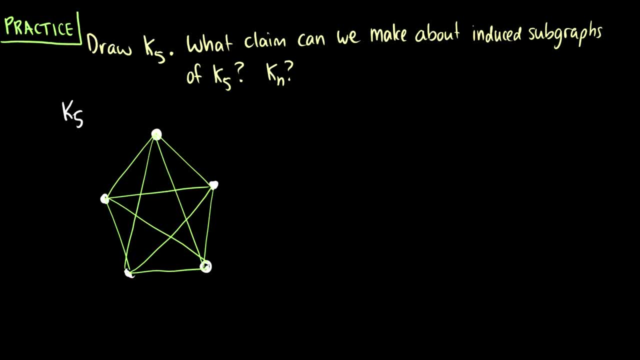 and we delete all adjacent edges. So let's, let's try this. Let's remove this vertex here and remove all incident edges. So this is k5 minus some vertex. What are we left with? We're left with k4, because each of these vertices are connected to three. 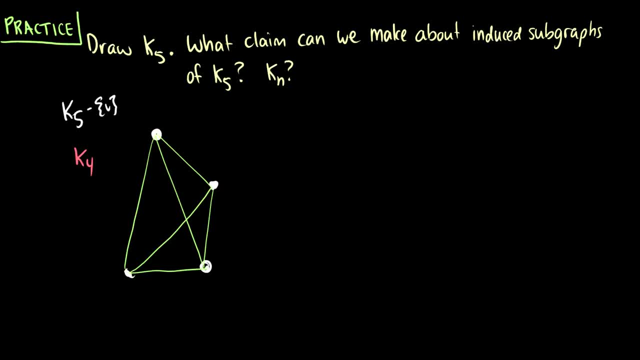 other vertices. Okay, so what happens if I remove another edge or another vertex? Well then, I remove, say, this one. Oh, what's that? We're now left with k3.. So what happens when we have kn and we remove a vertex? 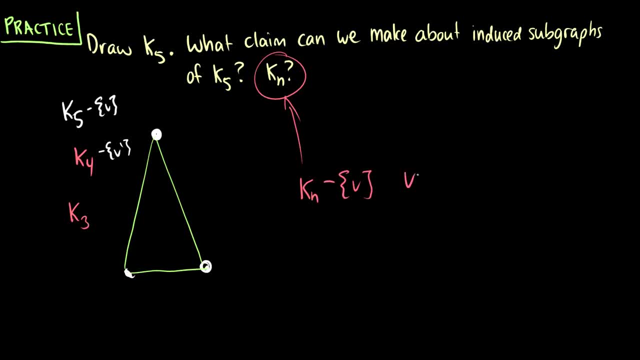 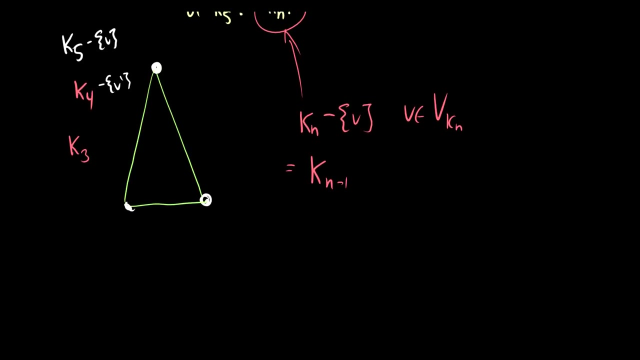 Well, if we take kn minus some random vertex for v in the vertex set of kn, then this is just equal to kn minus one, And we can keep going and going until we get back to k1.. So it's kind of interesting, In fact, when you say, okay, hold on a second, hold on a second. 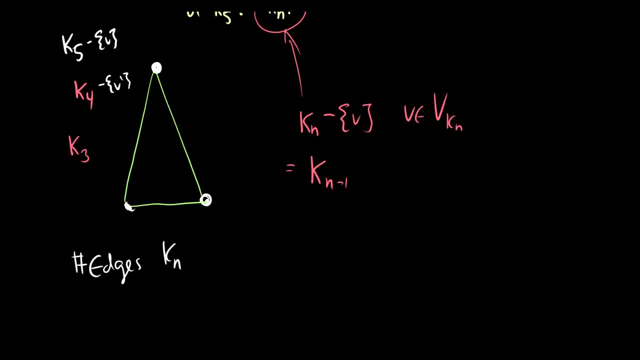 Let's take a look at the number of edges here in kn. Okay, so that's going to be n choose two, because we have n vertices and we choose two. So then what happens when we subtract? Okay, so that's n choose two. Now what do we get when we take the number of edges in kn, minus some vertex? 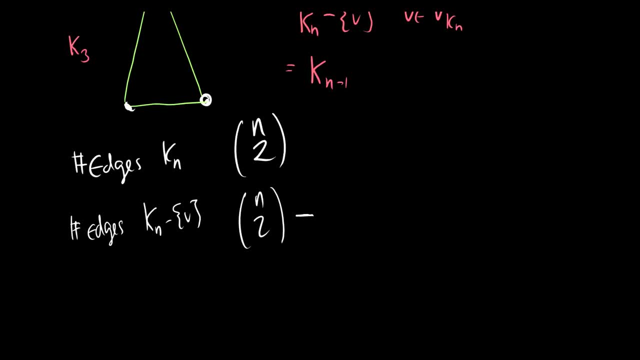 Well, we get n choose two, and then we subtract: Okay. so we pick a vertex, say here, and then it has to go to n minus one other vertices. So what happens is then we subtract n minus one edges, Okay. well, this is the same thing as n times n minus one over two minus n minus one. 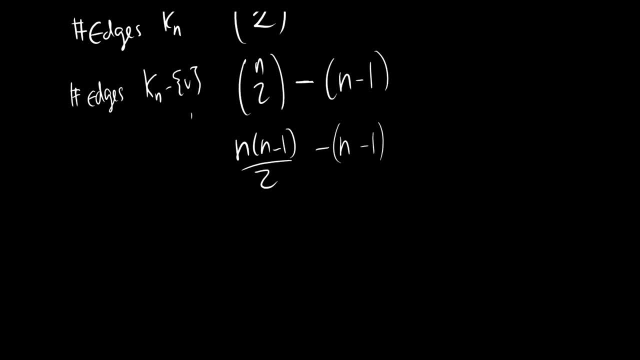 So well, what do we have here? We could put it all over the same common denominator. So this is going to be n times n minus one minus two, n plus two all over two. So this will be n squared minus n minus two, n plus two over two. 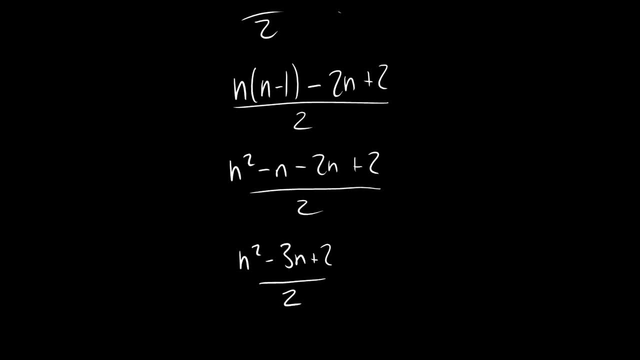 which is the same thing as n squared minus three, n plus two, all over two. And you're saying: hold on a second. this, this has to equal n minus one over two. What, what crazy shenanigans are you doing here? Well, let's take a look at this. 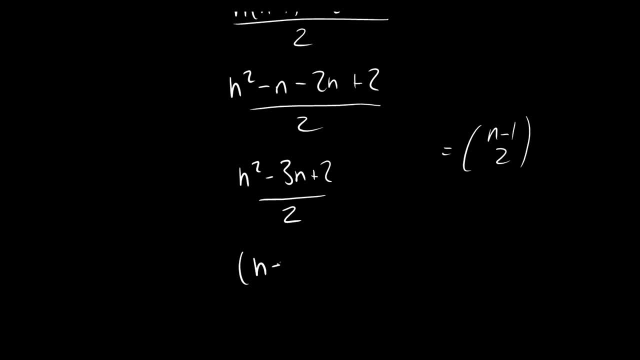 So we can factor this, this will be n minus two, n minus one all over two. Oh, so now you're sort of getting it right, and this is just the same thing as basically saying n minus two times n minus one times n minus three factorial over two times n minus three factorial. 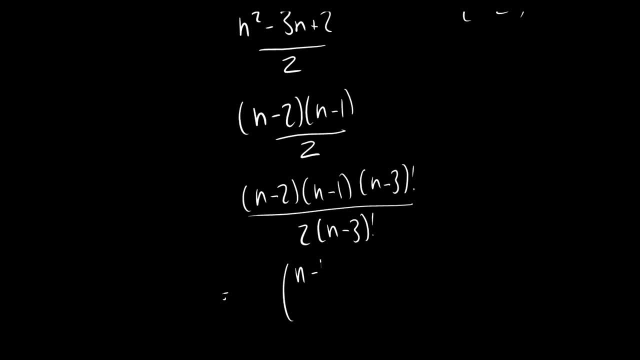 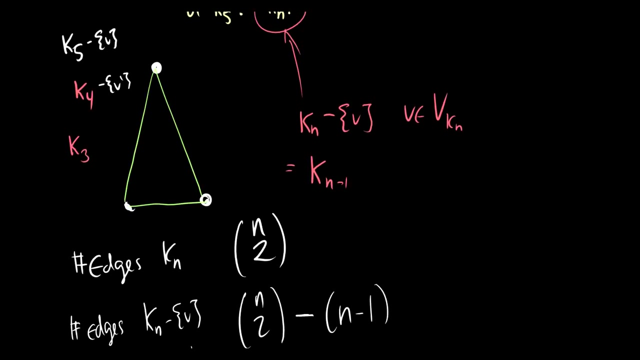 which is really just the same thing as saying: n minus one, choose two. So we have proven both graphically and mathematically that the number of edges in kn minus some vertex and all of its incident edges is equal to the number of edges in kn minus one.